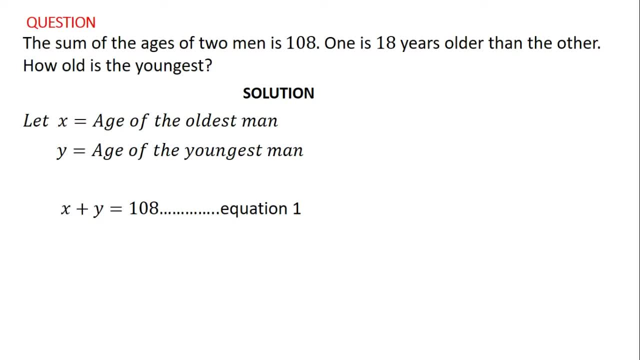 the question goes on to say that one is 18 years older than the other. one is 18 years older than the other. what that means is that if you subtract the age of the youngest man from the age of the oldest man, you are going to get 18, because if i'm 18 years older than you. what it means is that if 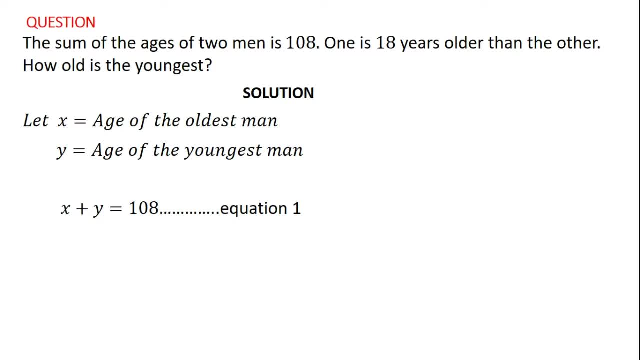 we take your age from my age, you are going to get 18. so the age of the youngest man is y. so if you subtract it from the age of the oldest man, which is x, you must get 18. so x minus y will give us 18. 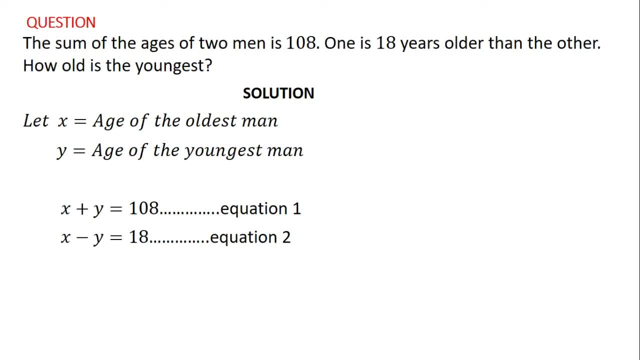 and that is equation two. now we have these two equations with two unknowns, so we can solve for x or y. okay, so let's go on. how do we solve for this? we have these two equations here. we've learned how to solve simultaneous linear equation. you can use any of the methods to solve it. 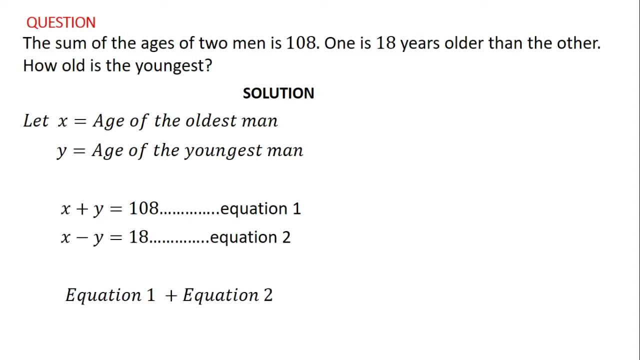 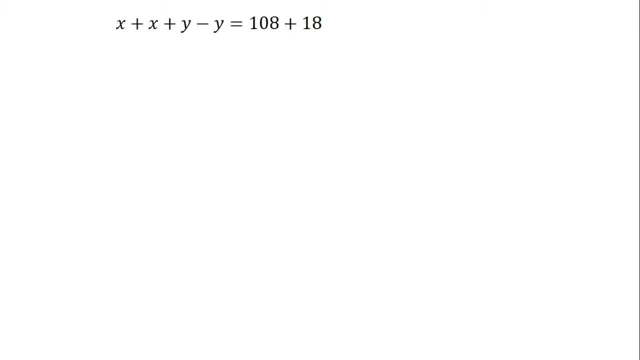 in this case i'm going to use the elimination method and i'll be eliminating y, so i'll add equation 1 to equation 2.. if i add equation 1 to equation 2, i will have x plus x plus y minus y is equal to 1, 0, 8 plus 18. so this will give me s plus s plus y minus y is equal to 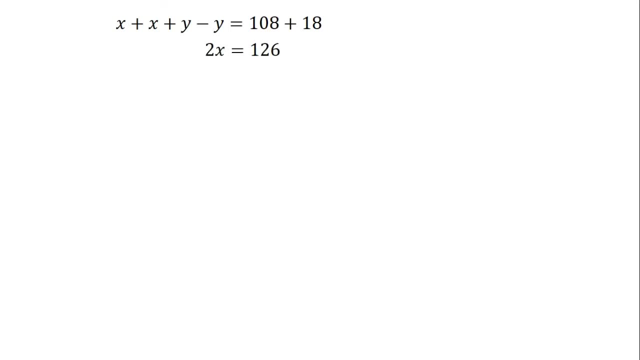 1, 0, 8 plus 18, y minus y will be 0 s plus x. from algebra we know that that is 2x and this is equal to 1, 26, because 8 1 0, 8 plus 18 will give us 1, 26.. okay, let's move on. 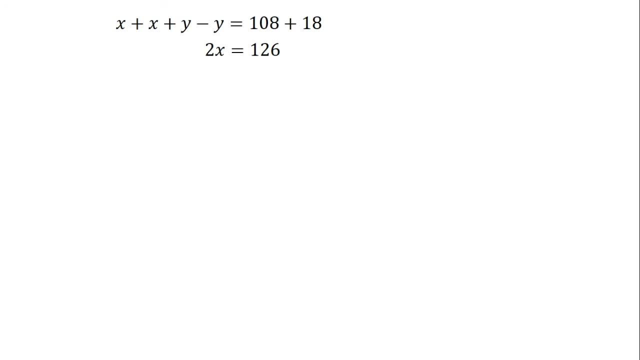 we are going to divide both sides by 2, so we divide the left hand side by 2 and we divide the right hand side by 2- we know this from linear equations- and x is going to give us 63. what that means is that the age of the oldest man is 63, or the oldest man is 63 years old. but the question? 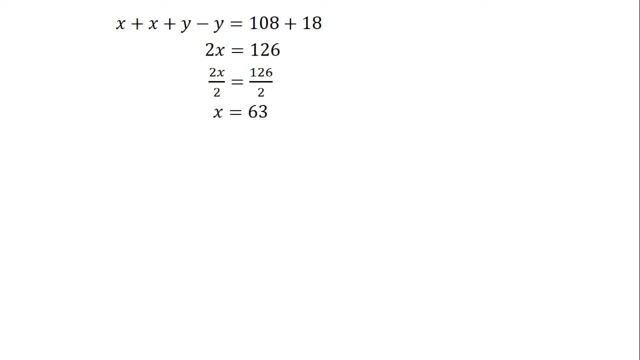 told us to find the age of the youngest man, which is y. and how do we do that? you pick one of the equations, so i'm picking equation one from equation one. we know that x plus y is equal to 1 0- 8, but we